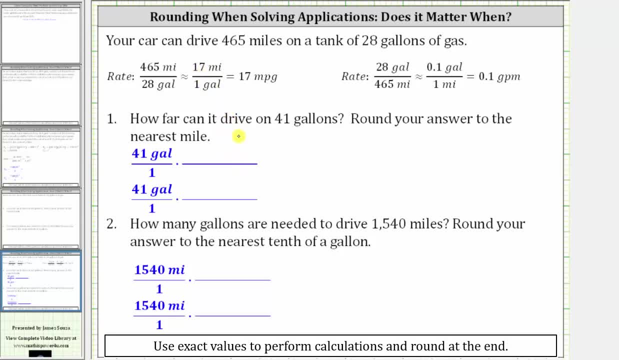 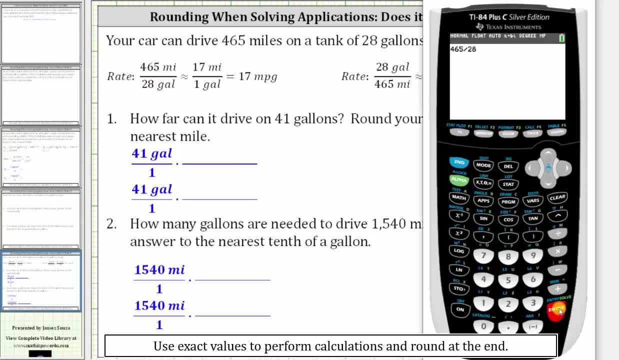 But again, we should avoid this because it gives us more of an error. But just for review, to find the unit rate in miles per gallon, we would divide 465 by 28,, which notice how, if we did round to the nearest mile, 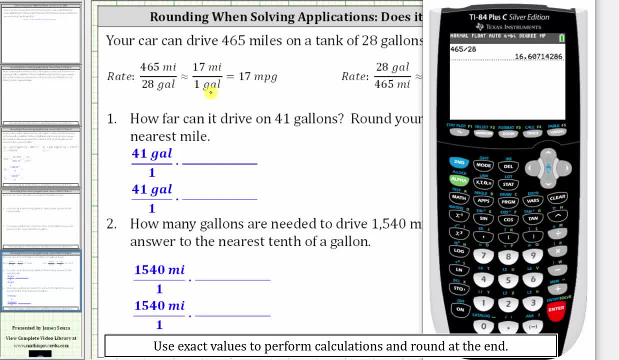 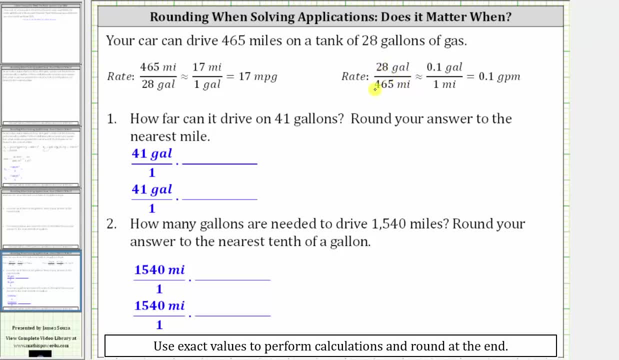 this would give us a unit rate of approximately 17 miles per one gallon, or 17 miles per gallon. To find the unit rate in gallons per mile, we divide 28 by 465.. If we did round to the nearest tenth, this would give us an approximate unit rate. 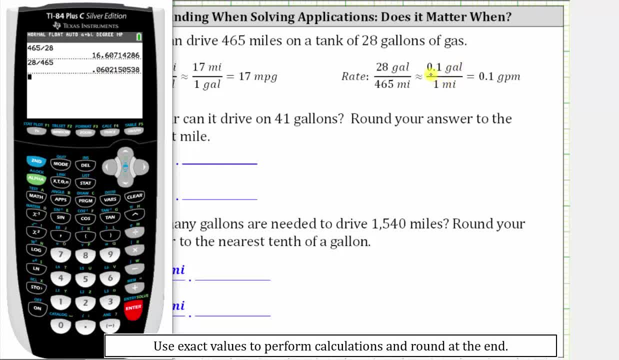 of 0.1 gallons per mile or 0.1 gallons per one mile, Notice how. because we have a six in the hundredths place value, we would round up to 0.1.. And now let's answer the two questions. 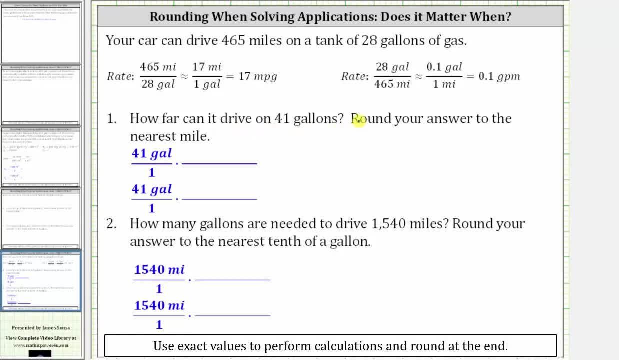 First, how far can the car drive on 41 gallons? To answer this question, we begin by writing 41 gallons as a fraction with the denominator of one. Because we want gallons to simplify out, we use the rate with gallons in the denominator. 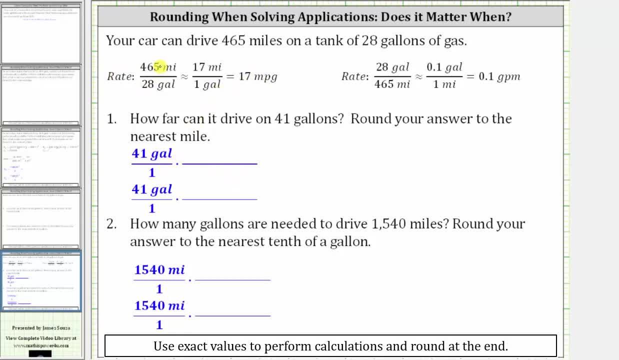 which would be this first rate here. So again, we should use the exact rate of 465 miles per 28 gallons. So again, we multiply by 465 miles over 28 gallons. Notice how the units of gallons simplify out, leaving us with 41 times 465,. 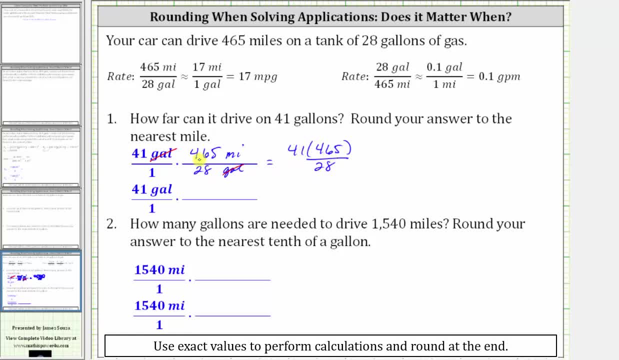 divided by 28,, and now the units are miles. So, again, this is the correct way to answer the question, because we are using the exact rate. And now going back to the calculator, we want to evaluate this quotient and then round to the nearest mile. 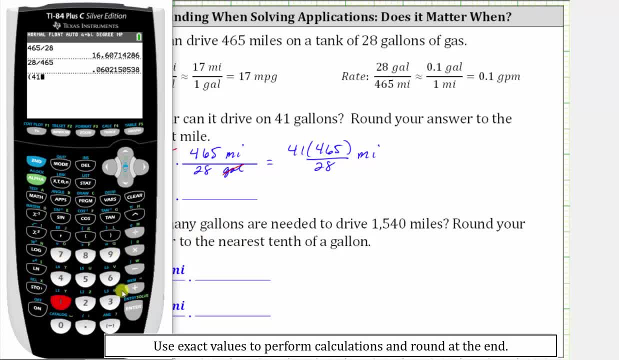 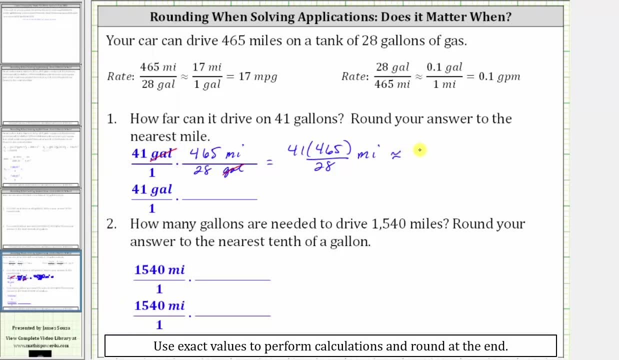 So we have, in parentheses, 41 times 465, and then divided by 28. Because we have an eight in the tenths place value round up to 681 miles. And now let's do it the incorrect way by using the rounded unit rate of 17 miles per one gallon. 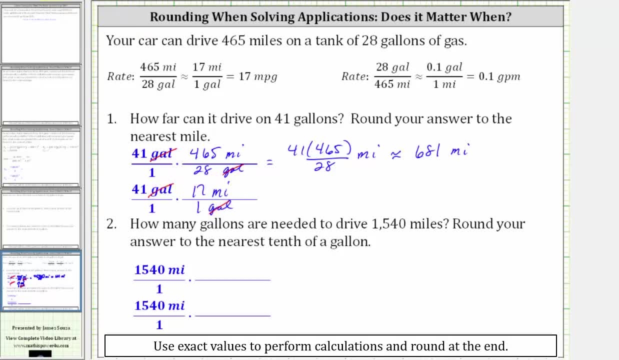 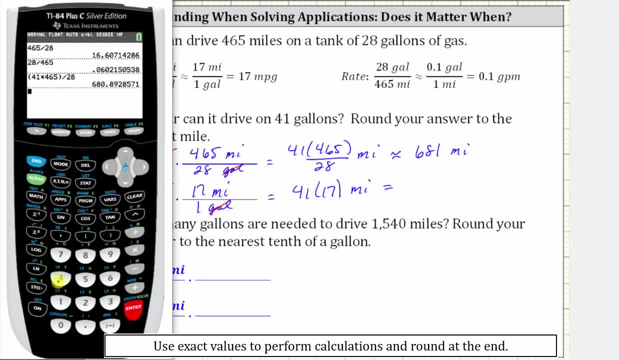 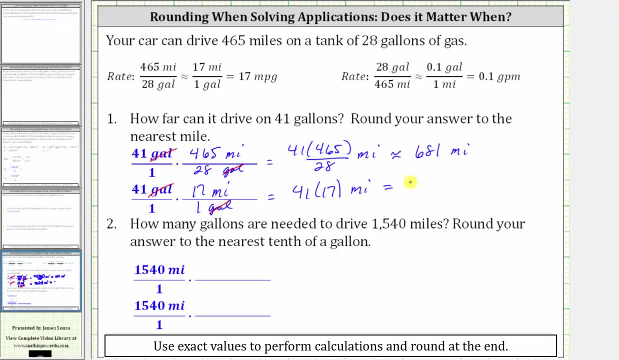 Again, notice how the units of gallons simplify out, leaving us with 41 times 17 miles. 41 times 17 is equal to 697 miles, So this estimate is not the estimate we should use, because it has much more of an error. 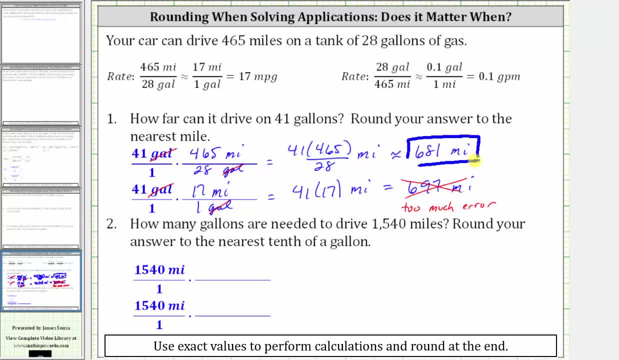 We should use the estimate of 681 miles, because we used the exact rate for the calculation. And now for number two: how many gallons are needed to drive 1,540 miles? We'll begin by writing this as a fraction, with a denominator of one. 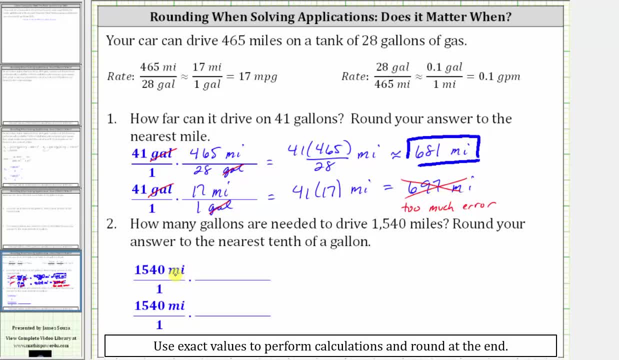 Because we want miles to simplify out, we use the rate with miles in the denominator, which is the second rate here. So the correct way is to use the exact rate of 28 gallons per 465 miles. Notice how the units of miles simplify out. 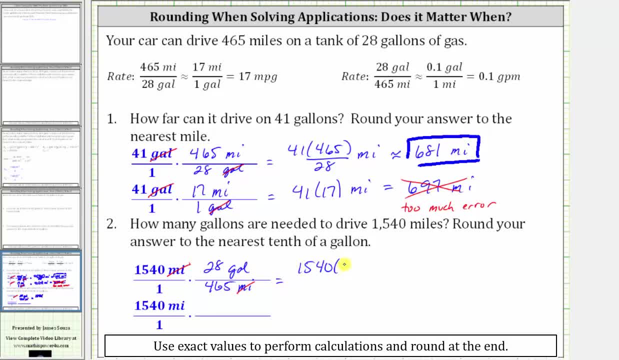 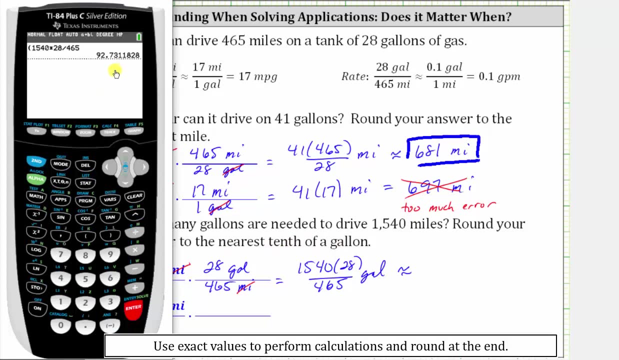 leaving us with 1,540 times 697 miles. So that's 28 times 28 divided by 465 gallons. And now we'll go back to the calculator and round this quotient to the nearest 10th of a gallon, Because we have a three in the hundredths place value. 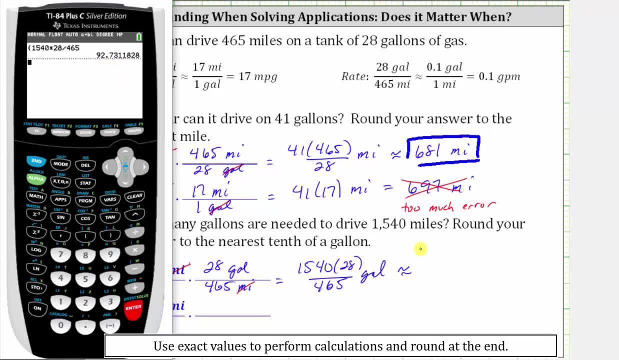 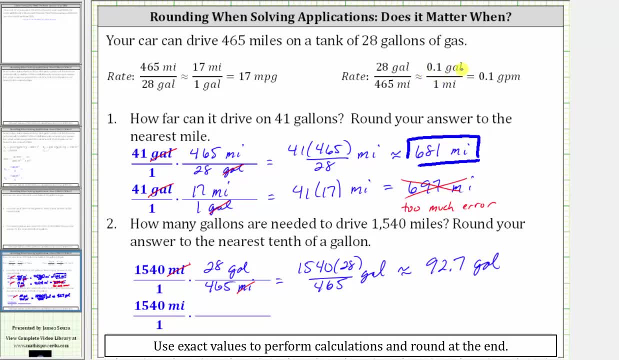 we round down to 92.7 gallons. And now let's answer the question again and use the rounded rate of 0.1 gallons per one mile. This is the way we should not do it, but we can do it Because we are going to have more of an error. 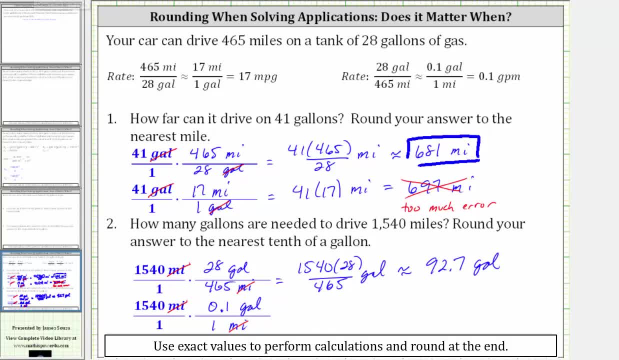 Notice how the units of miles simplify out, which leaves us with 1,540 times 0.1 gallons. 1,540 times 0.1 is equal to 154.. Notice how we have a big difference between the number of gallons needed to drive 1,540 miles. 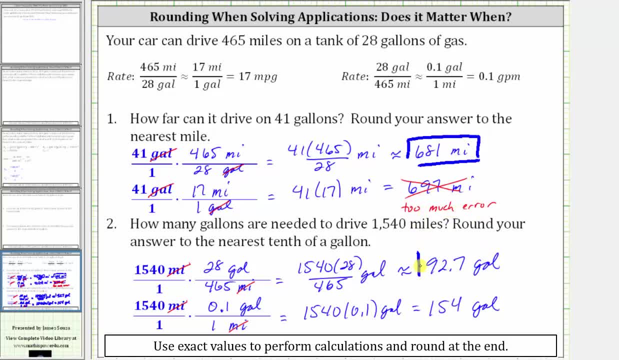 Our correct estimate should be approximately 92.7 gallons. It should not be 154 gallons because we used the rounded rate to perform this calculation. The estimate of 154 gallons has too much error. I hope you found this helpful.